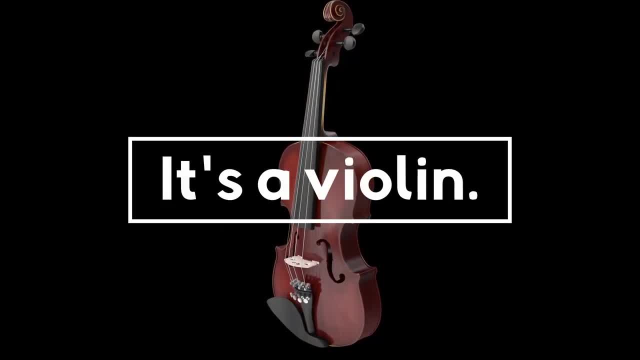 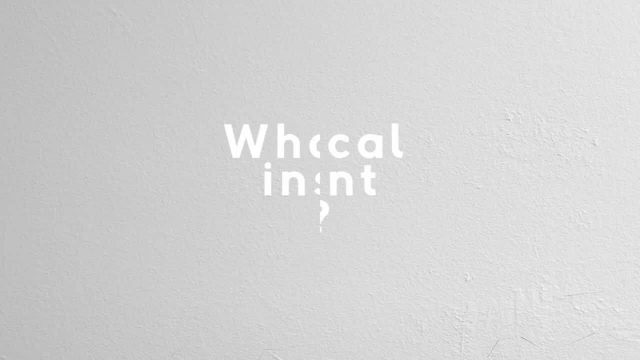 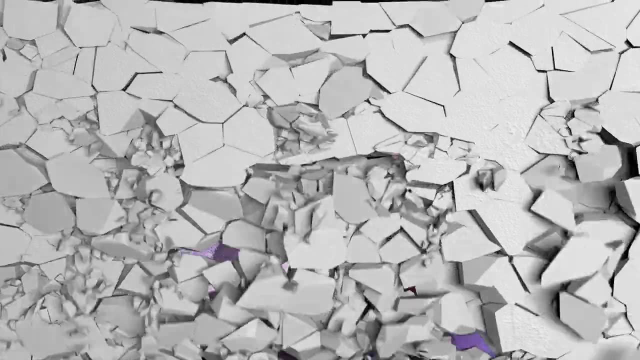 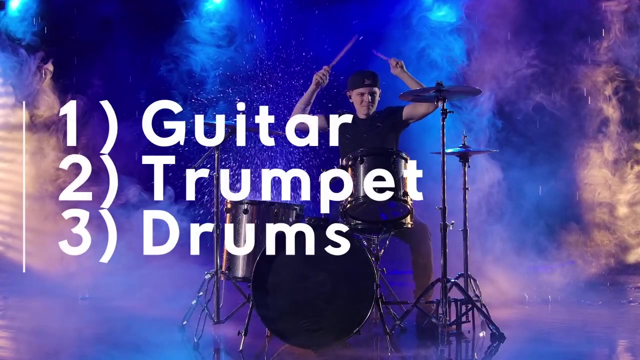 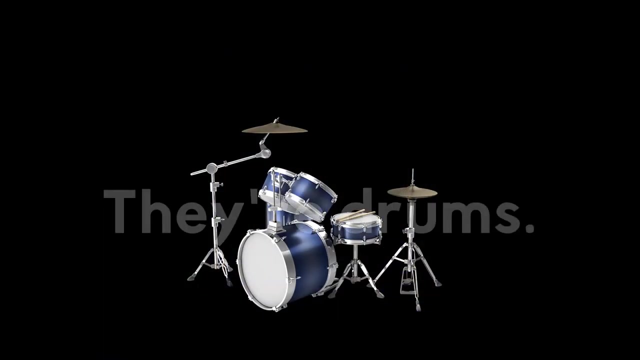 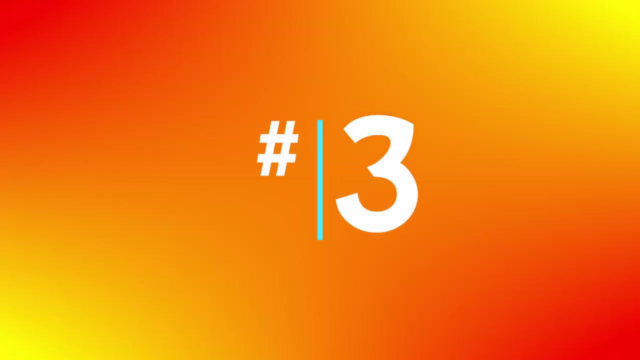 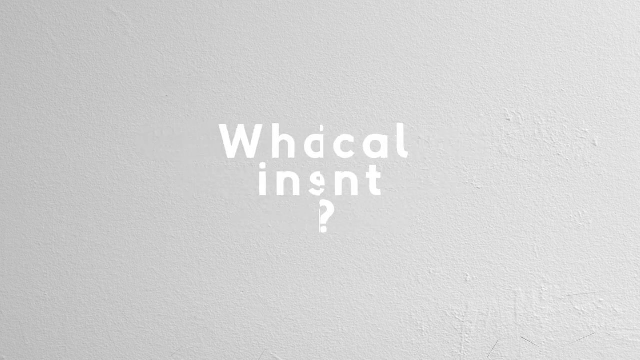 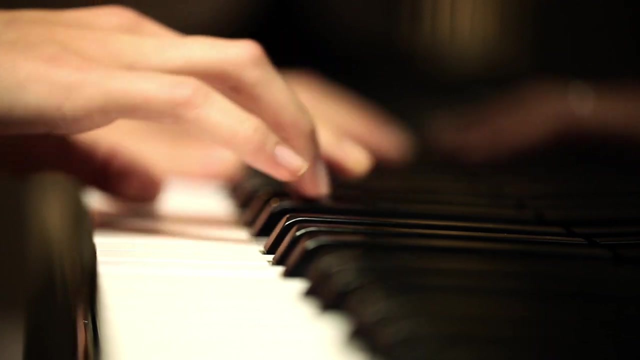 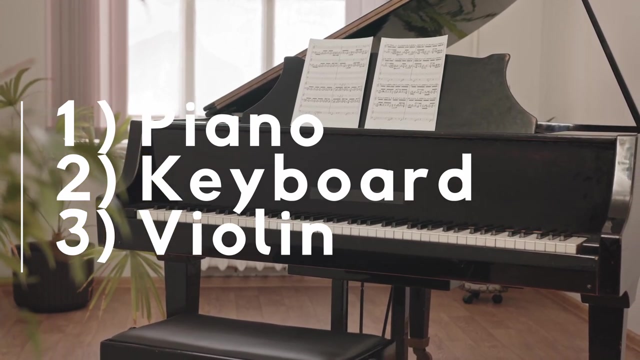 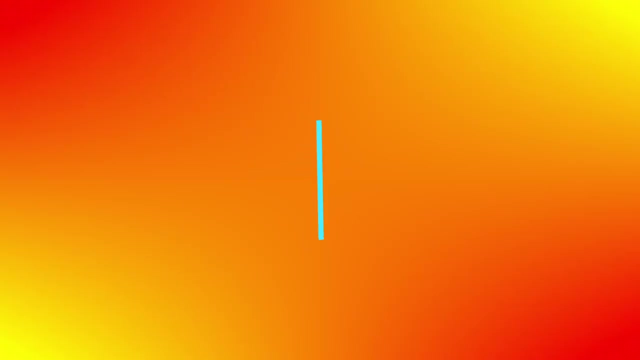 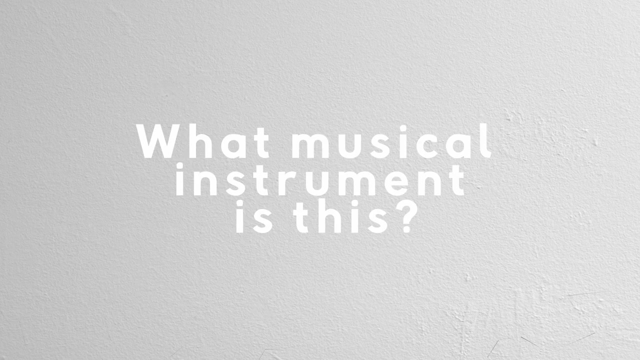 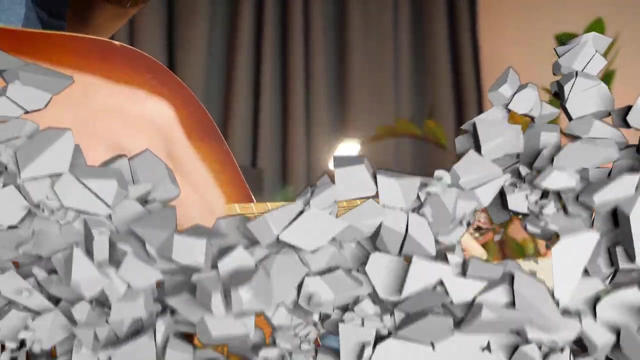 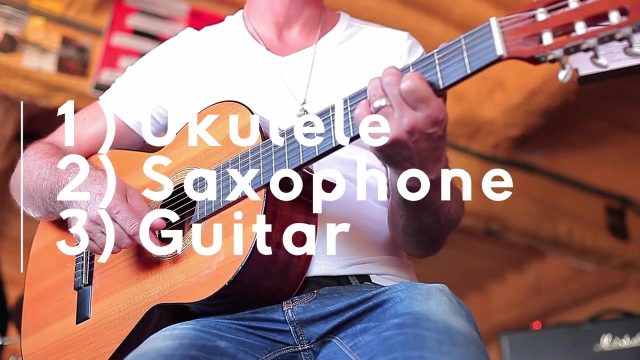 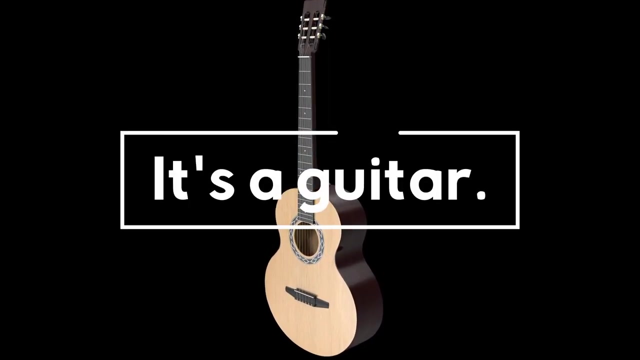 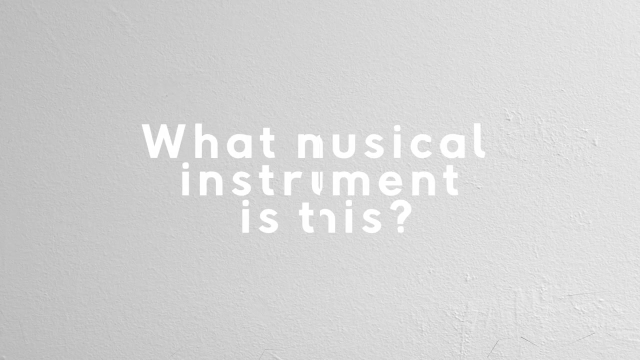 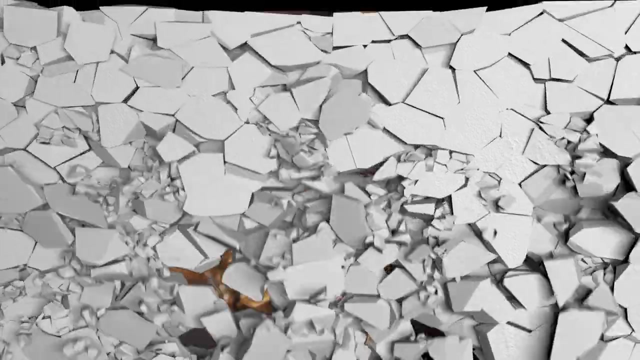 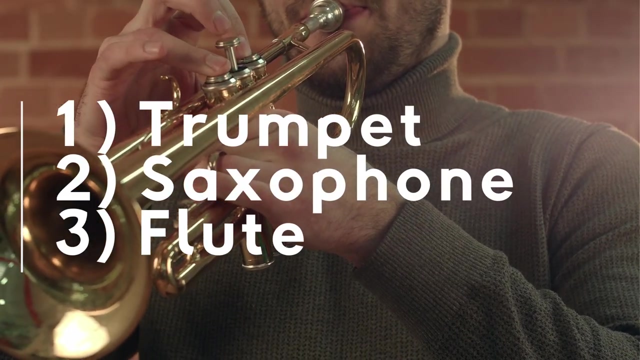 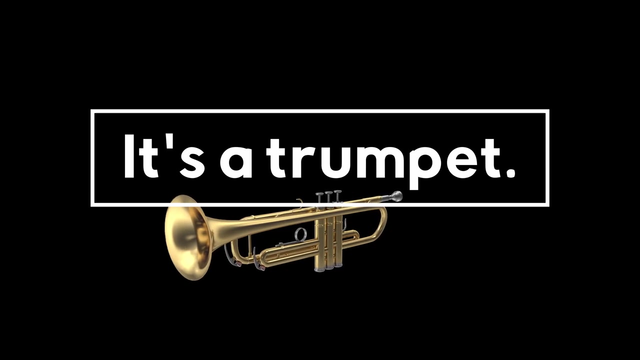 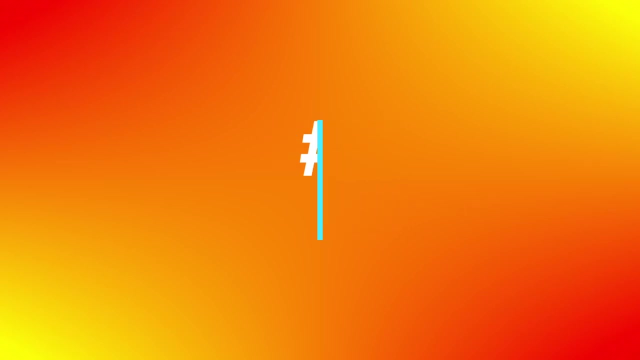 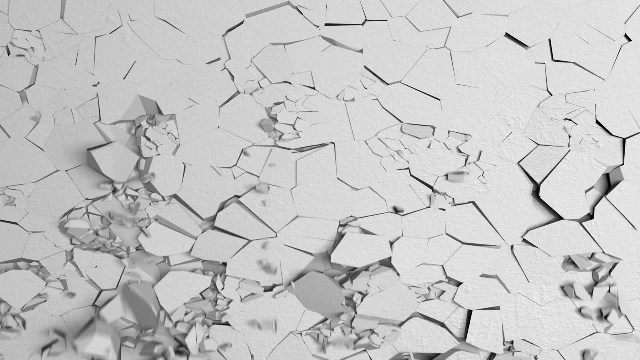 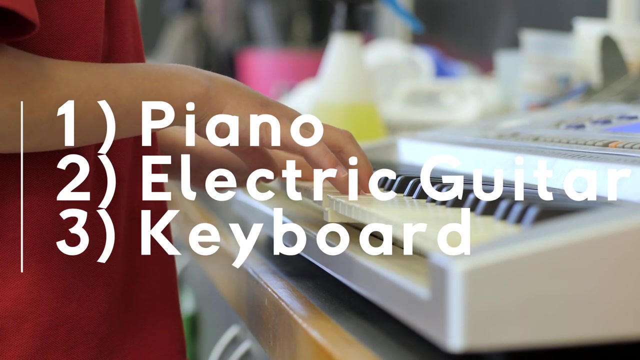 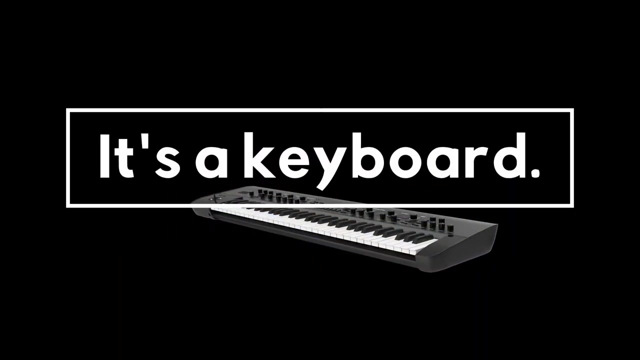 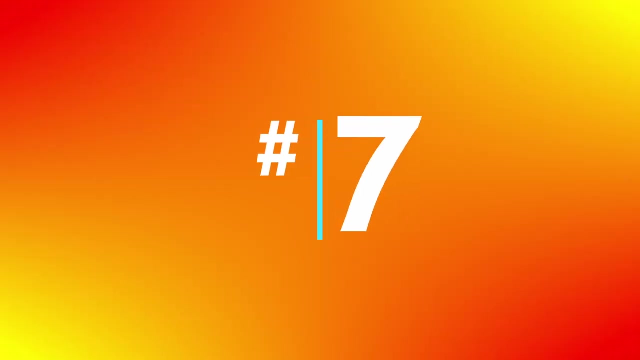 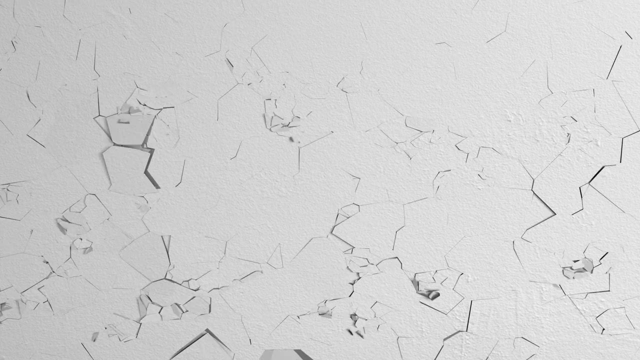 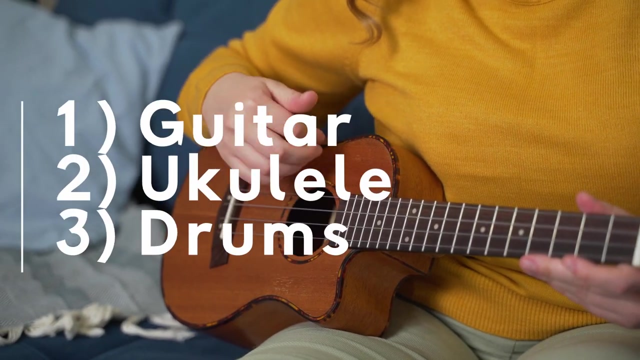 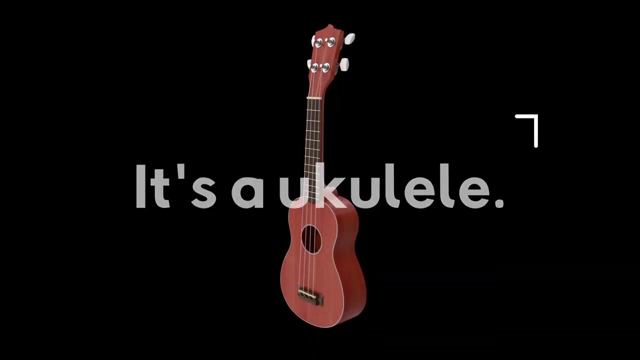 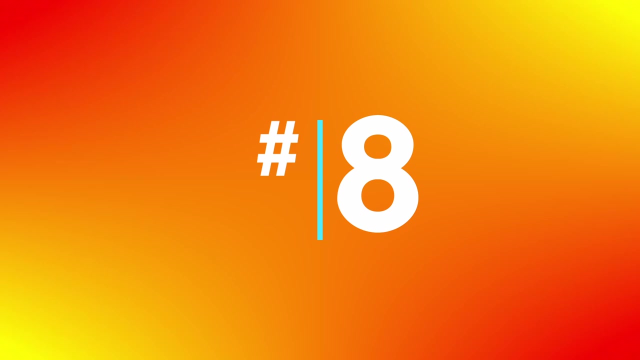 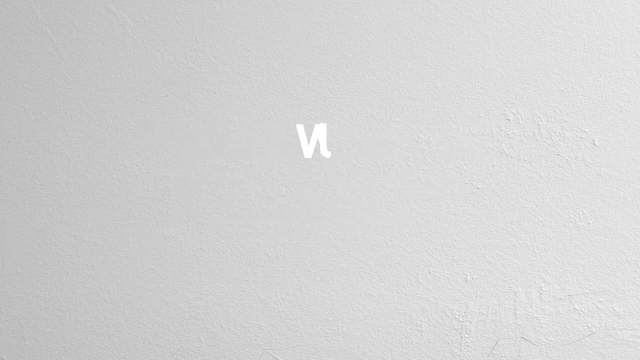 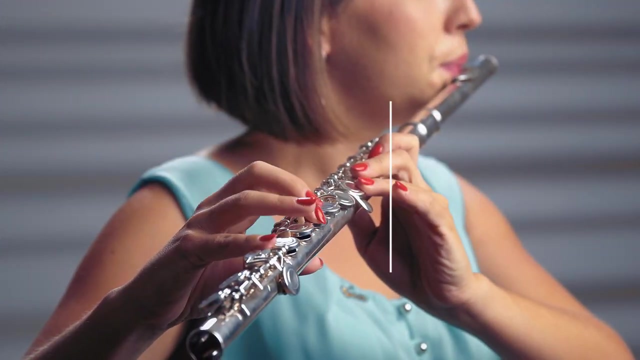 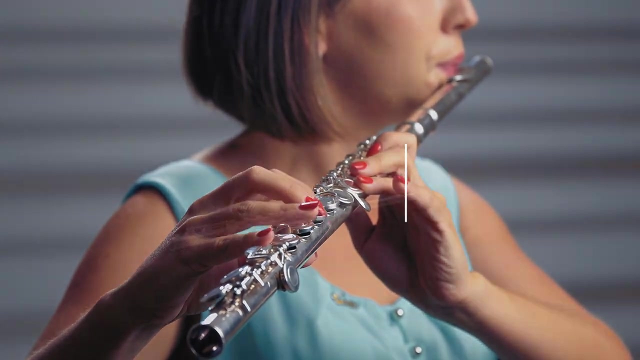 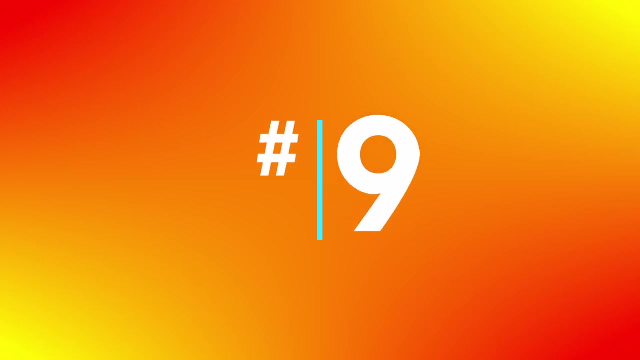 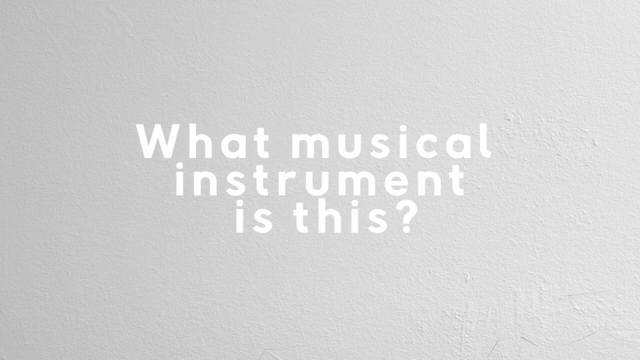 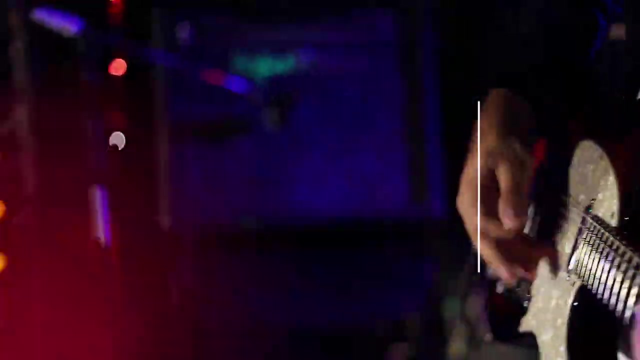 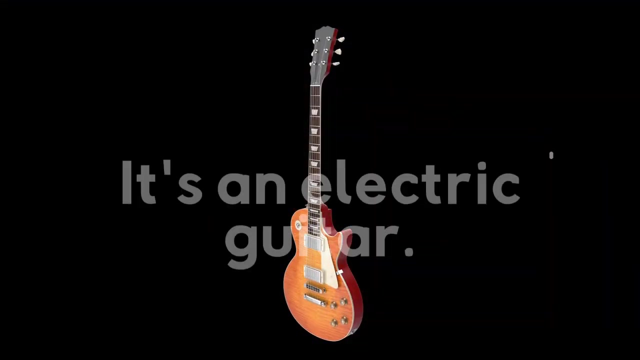 Thank you for watching. Thank you for watching. They're drums. It's a piano. It's a guitar. It's a trumpet. It's a keyboard. It's a ukulele. It's a flute. It's an electric guitar.